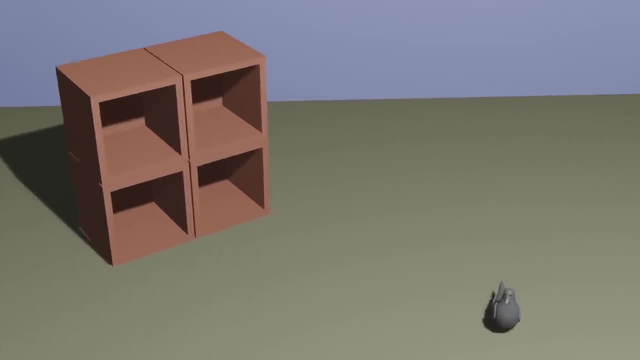 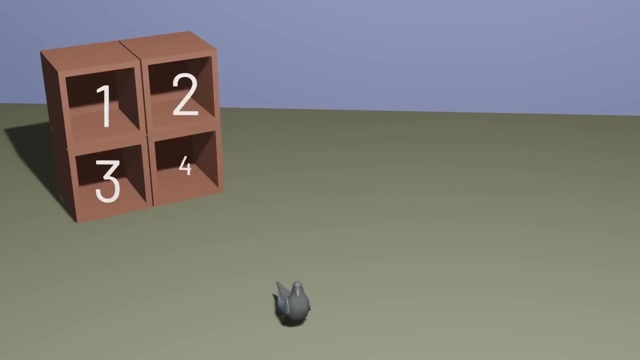 The pigeonhole principle is one of those ideas that sounds completely obvious but turns out to be pretty useful. Here's the idea: Let's say there are four pigeonholes, and let's also say we have five pigeons, each of which needs to be put into one of those holes. 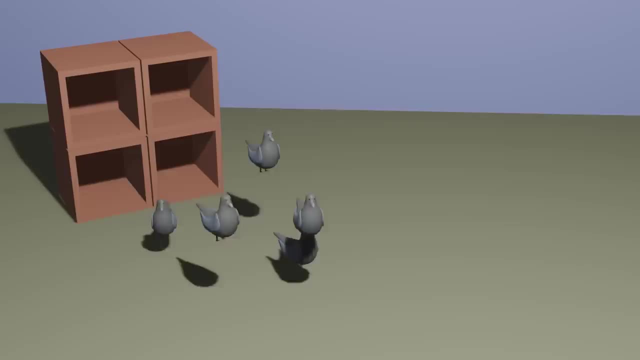 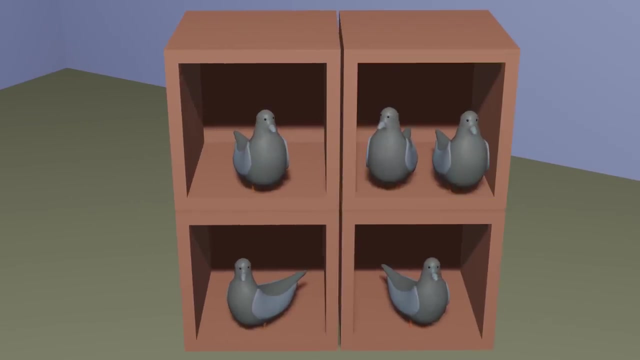 The pigeonhole principle says that after we've put each pigeon into a pigeonhole, there must be at least one pigeonhole that has multiple pigeons in it, And that's it. That's the whole idea, Or I suppose, to state the principle a little more generally. 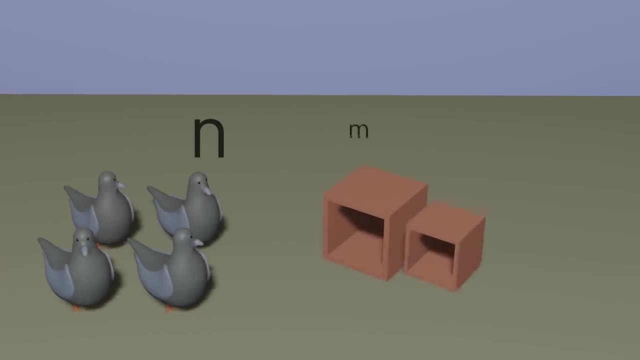 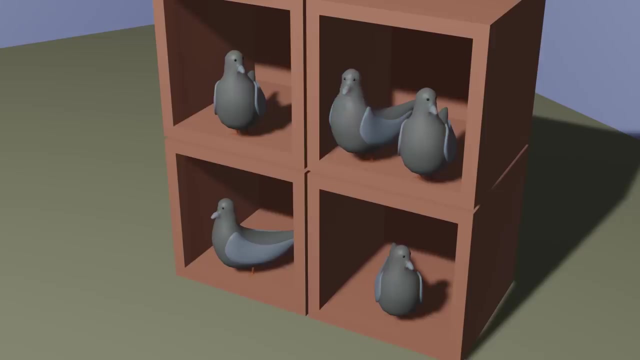 if we have n pigeons put into m pigeonholes and n is greater than m, then there must be at least one pigeonhole that contains more than one pigeon. When I first heard this principle, it just sounded obvious and I wondered how an idea. 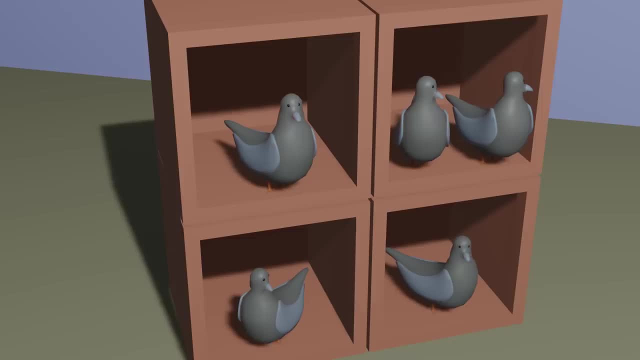 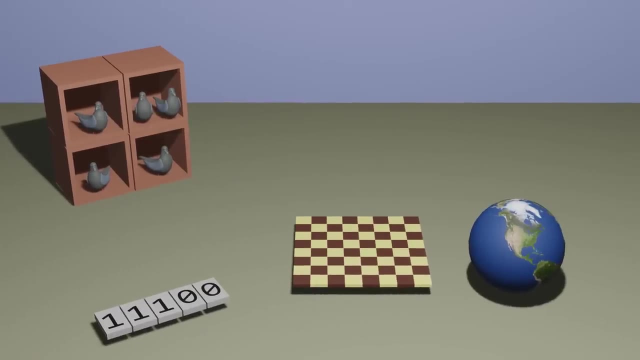 so straightforward and trivial could actually prove practical. But it turns out a lot of problems of pigeonhole principle are based on how we think of pigeonholes And so, for example, have solutions that in whole or in part can be answered by applying the pigeonhole. 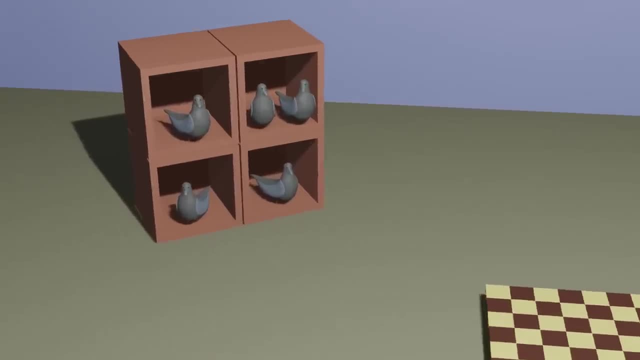 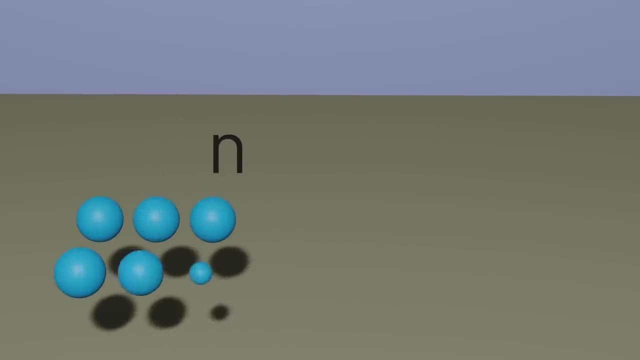 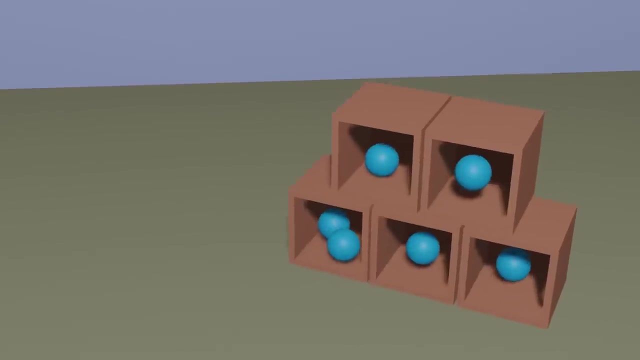 principle. Of course, usually we're not literally talking about pigeons and pigeonholes, but instead talking more generally about any objects. If we distribute n items across m groups and there are more items than there are groups, then at least one of those groups must have more than one item in it. 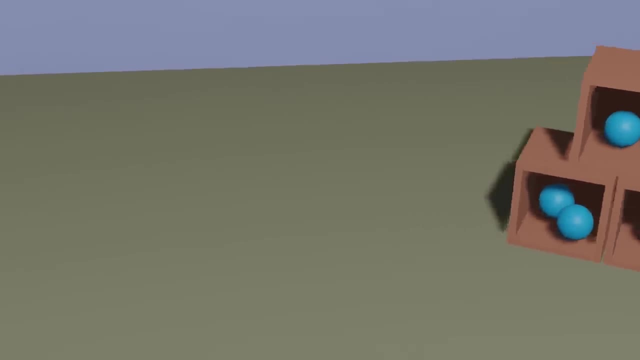 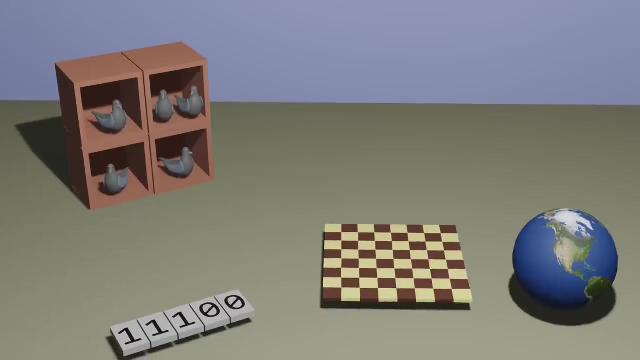 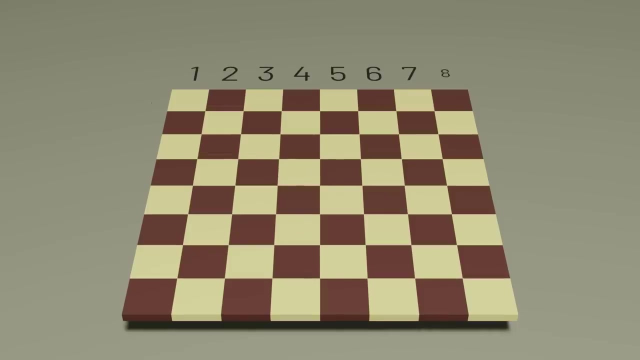 Solving certain problems then just comes down to identifying what our pigeons and pigeonholes actually are. So today let's take a look at some interesting applications of the pigeonhole principle, and let's start with a puzzle. Say, we have a chessboard, an 8x8 grid of alternating. 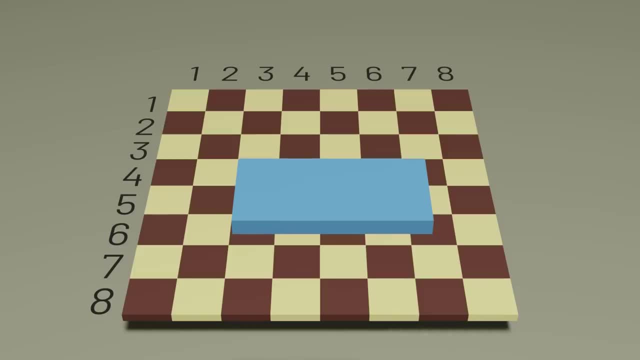 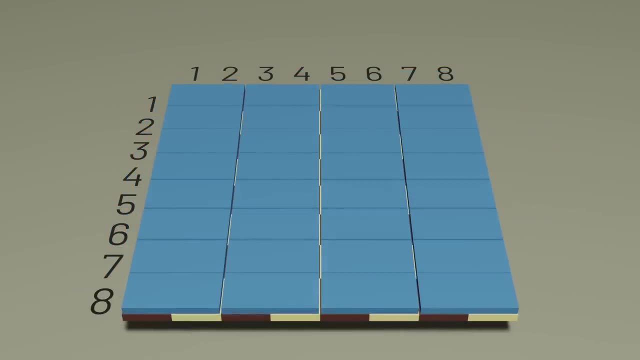 light and dark squares. If we take dominoes, each of which can cover up two of these squares, we can lay them out in such a way that they perfectly tile this chessboard. That's not too much of a surprise. There are 64 squares on the 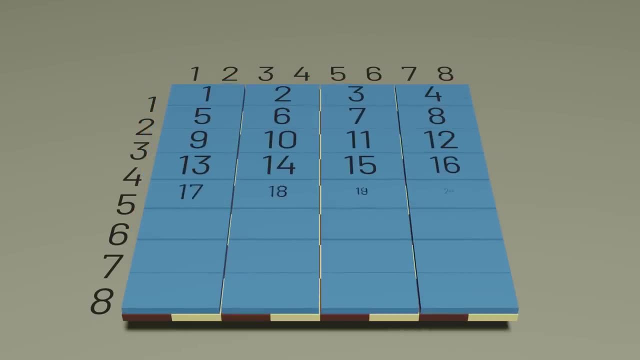 chessboard and here we're using 32 dominoes to cover the whole board perfectly, With no dominoes sticking out, no square left uncovered and no square covered twice. If we remove one square from this chessboard, it's pretty clear. 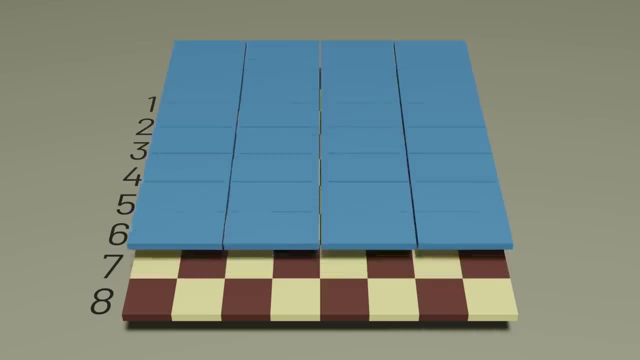 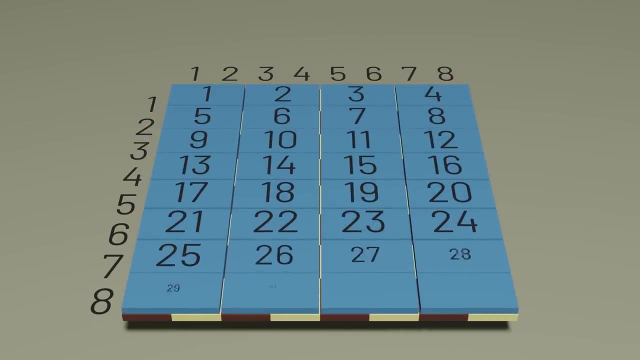 this chessboard. That's not too much of a surprise. There are 64 squares on the chessboard and here we're using 32 dominoes to cover the whole board perfectly, With no dominoes sticking out, no square left uncovered and no square. 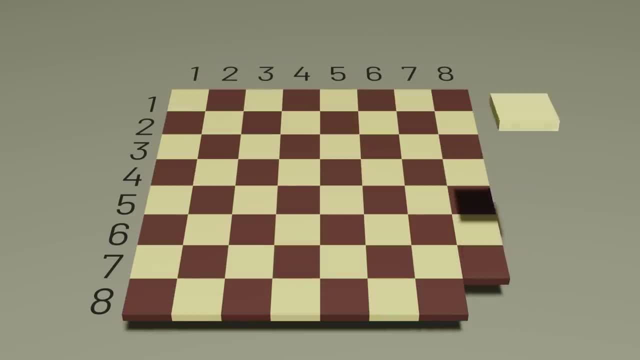 covered twice. If we remove one square from this chessboard, it's pretty clear that it's now impossible to tile the board. There's an odd number of squares, but using dominoes we could only ever cover an even number of squares. But what? 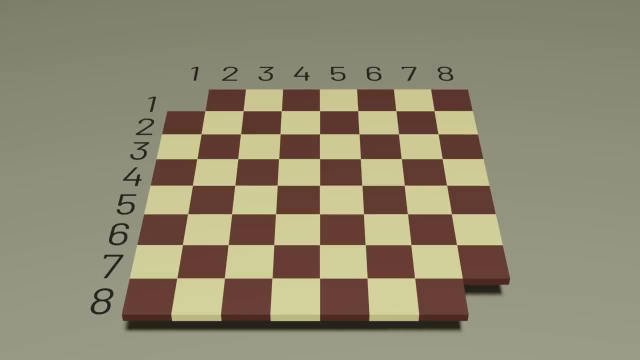 if we removed two squares from the chessboard from opposite corners of the board, Is it still possible to tile this board perfectly? It might not be so clear at first and you can try it, attempting to lay out tiles in just the right. 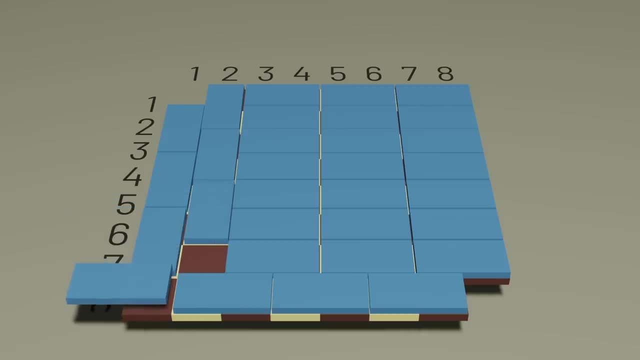 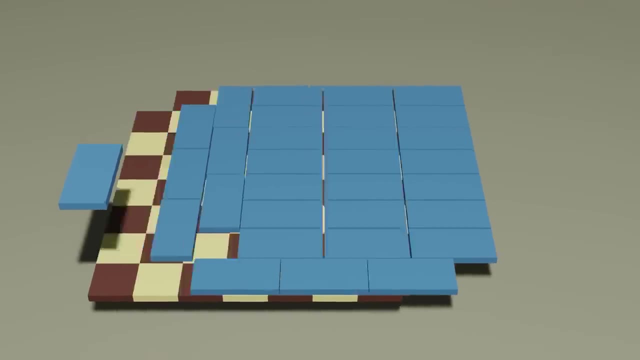 places, but ultimately you'll find that you won't be able to Perfectly tiling this board with dominoes isn't possible. But how do we know? Well, to tile 62 squares, we would need 31 dominoes And 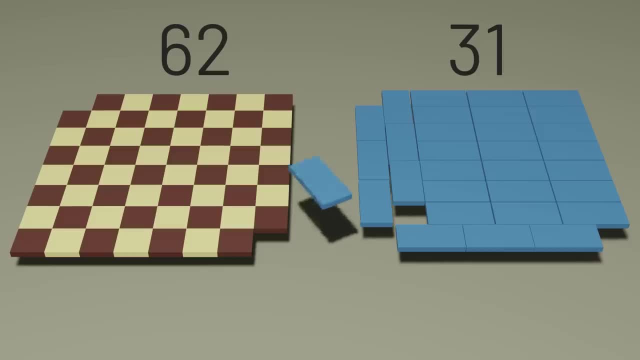 importantly, when each domino is laid on the board, it's going to cover up two squares, One dark square and one light square. no matter how that domino is oriented And how many light squares are on this chessboard anyways, Well, a full. 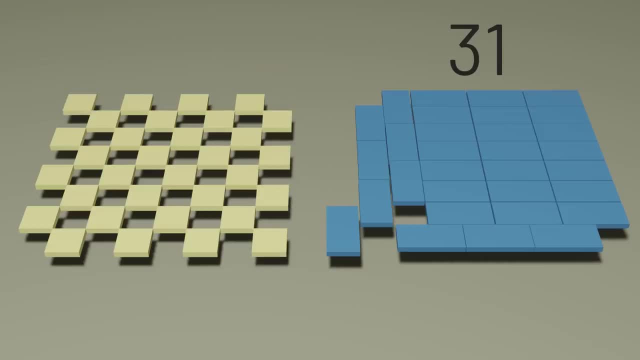 chessboard has 32 light squares, But since we removed two light squares from opposite corners of this board, we now have 30 light squares. See where this is going. We can now apply the pigeonhole principle. Our pigeons are the 31 dominoes and our pigeonholes are the 30 light squares Each domino needs. 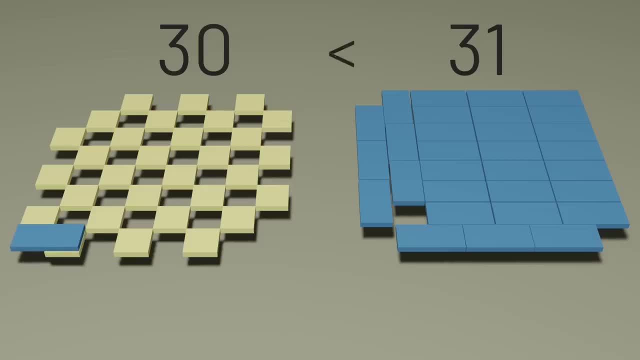 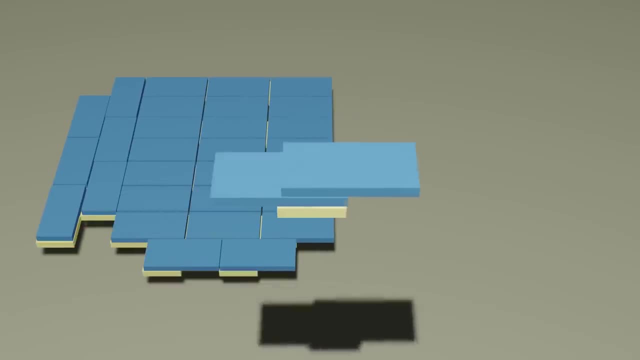 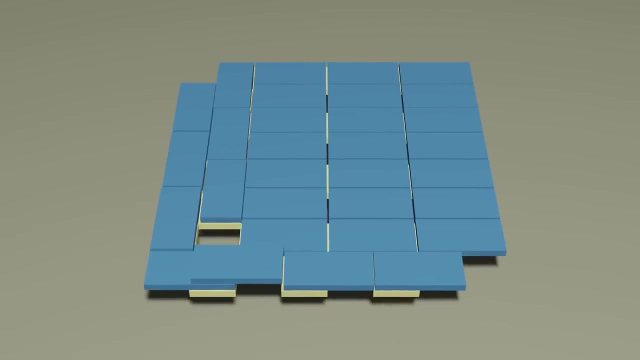 to cover one of the light squares And since we have more dominoes than light squares, there therefore must ultimately be at least one light square covered by multiple dominoes, And since, in a perfect tiling, each square should be covered by exactly one domino, we can therefore say that a perfect tiling isn't possible. 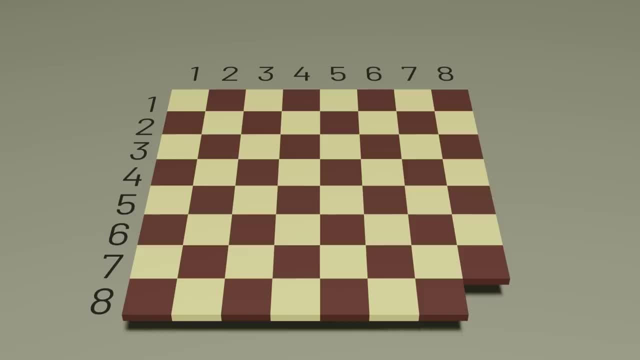 that it's now impossible to tile the board. There's an odd number of squares. but using dominoes we could only ever cover an even number of squares. But what if we removed two squares from the chessboard from opposite corners of the? 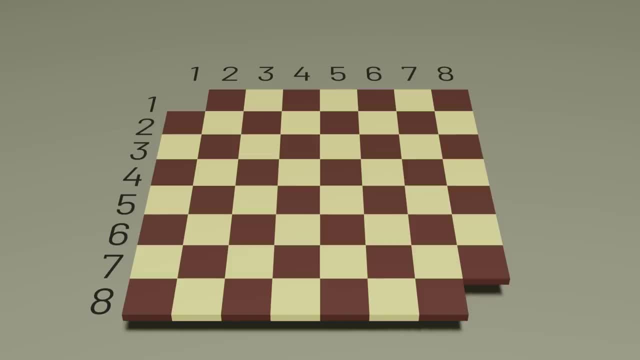 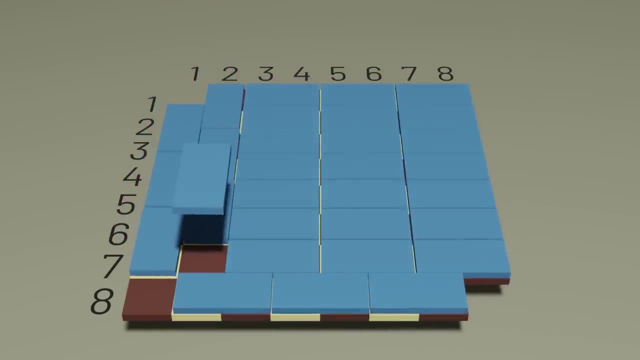 board. Is it still possible to tile this board perfectly? It might not be so clear at first and you can try it, attempting to lay out tiles in just the right places, but ultimately you'll find that you won't be able to Perfectly tiling. 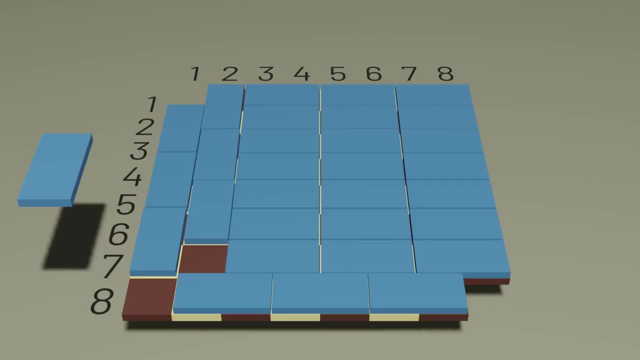 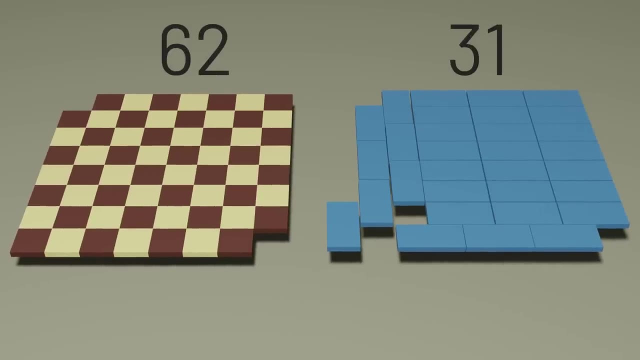 this board with dominoes isn't possible. But how do we know? Well, to tile 62 squares we would need 31 dominoes And, importantly, when each domino is laid on the board, it's going to cover up two squares: One dark square and one light. 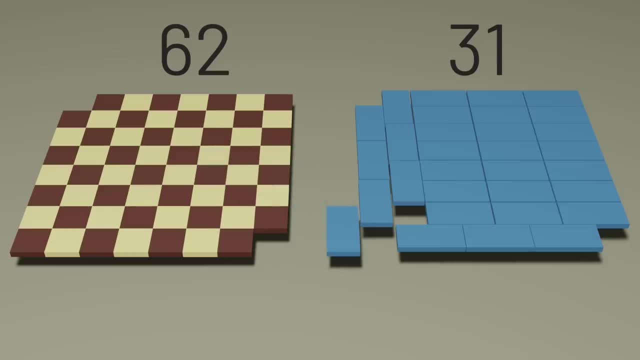 square, no matter how that domino is oriented And how many light squares are on this chessboard anyways. Well, a full chessboard has 32 light squares and But since we removed two light squares from opposite corners of this board, we now have 30 light squares. 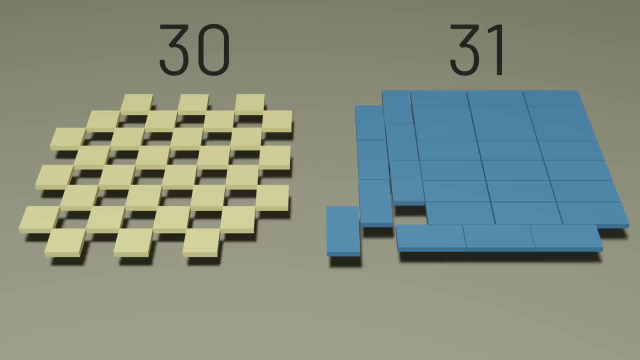 See where this is going. We can now apply the pigeonhole principle. Our pigeons are the 31 dominoes and our pigeonholes are the 30 light squares. Each domino needs to cover one of the light squares And, since we have more dominoes than light squares, there therefore must ultimately be at least one light square covered by multiple dominoes. 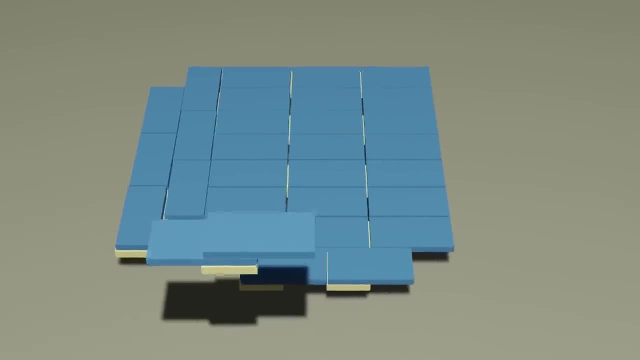 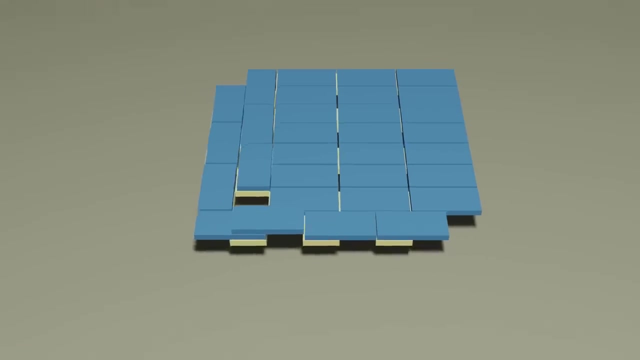 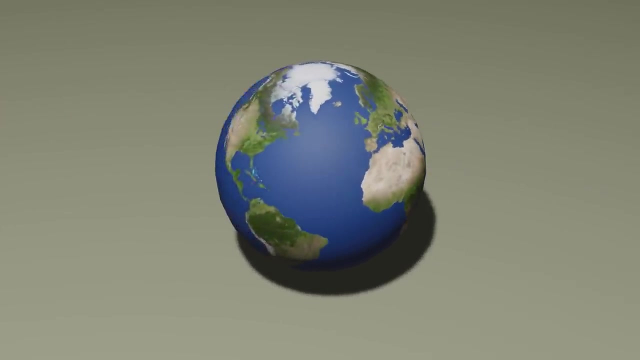 And since, in a perfect tiling, each square should be covered by exactly one domino, we can therefore say that a perfect tiling isn't possible. Let's take a look at another example. Let's imagine planet Earth, which, for simplicity, we'll here assume is a perfect square. 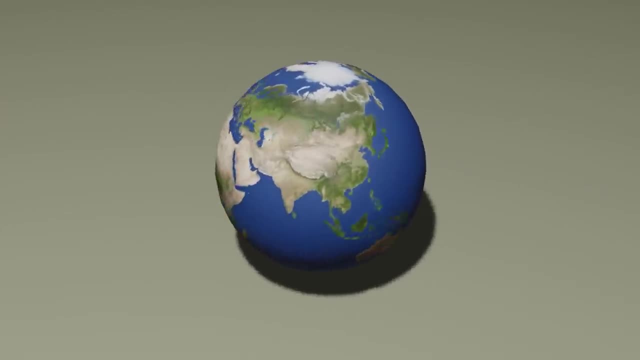 Let's take a look at another example. Let's imagine planet Earth which, for simplicity, we'll here assume is a perfect sphere. Earth can be divided into a northern hemisphere and a southern hemisphere, but that's not the only way to divide the Earth into two. 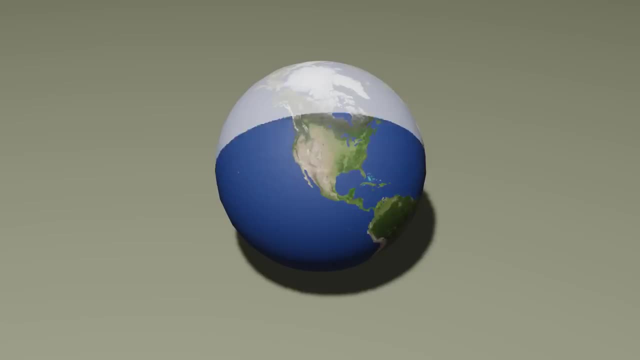 pieces. A hemisphere is just any half of the sphere, And a closed hemisphere is a hemisphere that includes the dividing line between the two halves. So now here's the question: If you pick any five points on Earth, can you find some closed hemisphere that includes at least four of those five points? 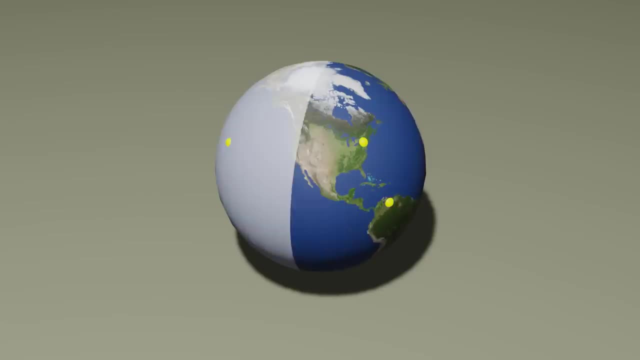 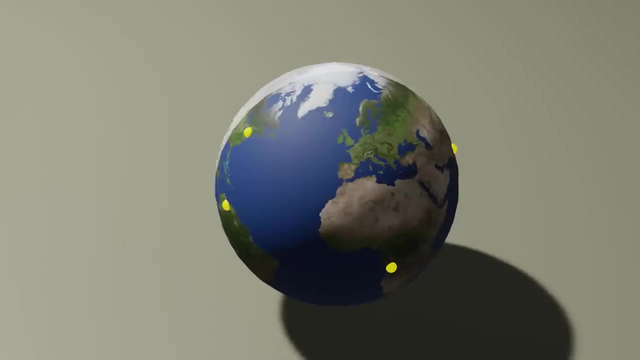 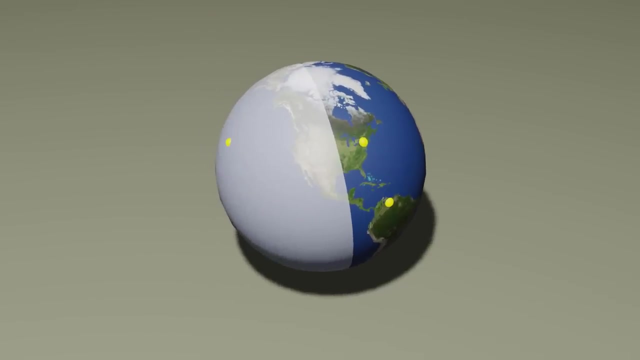 We can try an example: We pick five points at random and try some different hemispheres, And in this case we can eventually find a hemisphere that contains four of those five points. But will that always be the case? It turns out the answer is yes. We can start by saying that with any two points on Earth, 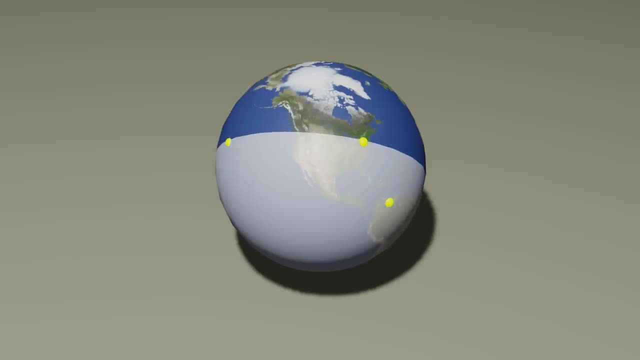 we can use those two points as the dividing line between hemispheres. After that, we're left with three remaining points, each of which must belong to one of these two hemispheres. Do you see where the opportunity for the pigeonhole principle? 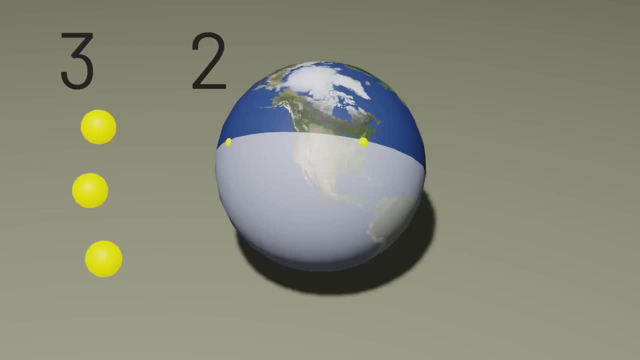 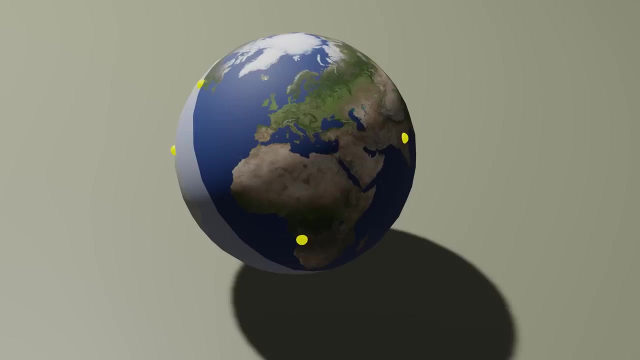 is If we let the points be our pigeons and the hemispheres be our pigeonholes. look what happens. We have more points than hemispheres, so there must be some hemisphere that has at least two points. And if that hemisphere has at least two of these points, plus the 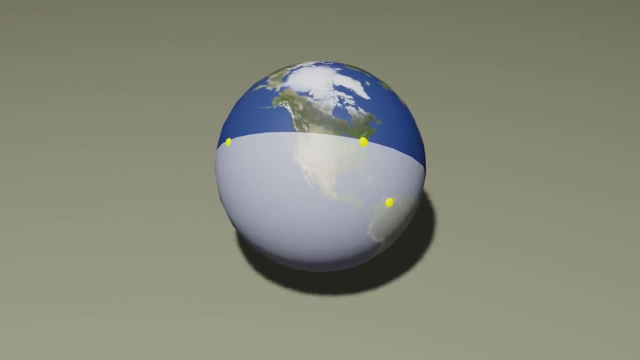 two points on the dividing line, then it therefore contains four out of the five points. So for any five places on Earth, four of them will always be on the same half of the planet, proven by the pigeonhole principle. And the pigeonhole principle isn't just useful for solving puzzles, It has practical 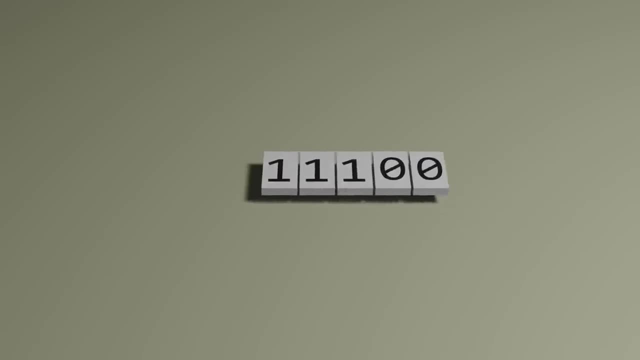 computational consequences too. One natural extension of the principle has to do with compression, converting some longer representation of data to some shorter representation. There's a particular form of compression called lossless compression, where, as the name suggests, no information is lost in the compression process. In other words, once we have the 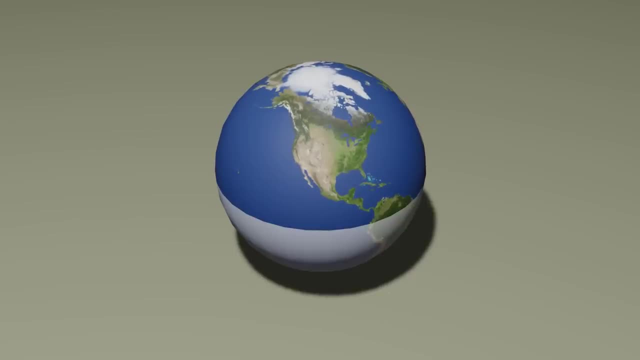 Earth can be divided into a northern hemisphere and a southern hemisphere, but that's not the only way to divide the Earth into two pieces. A hemisphere is just any half of the sphere, And a closed hemisphere is a hemisphere that includes the dividing line between the two halves. 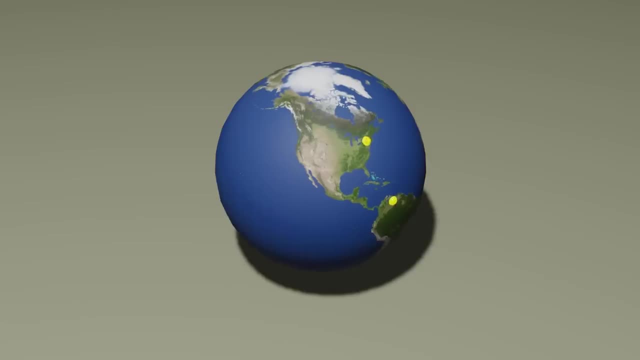 So now here's the question: If you pick any five points on Earth, can you find some closed hemisphere that includes at least one domino? If you pick any five points on Earth, can you find some closed hemisphere that includes at least four of those five points? 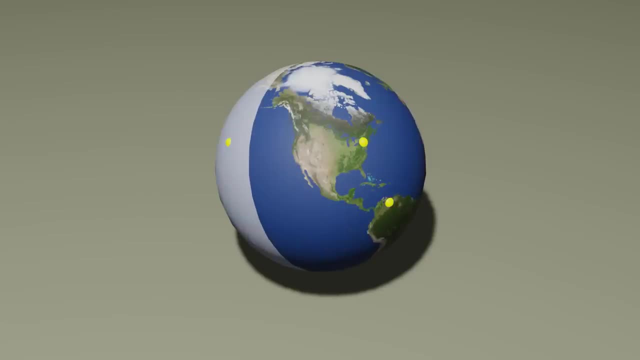 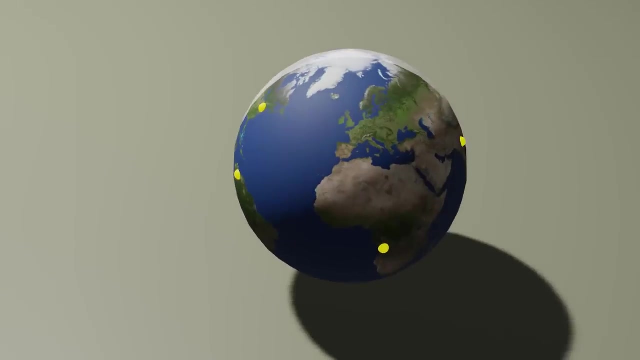 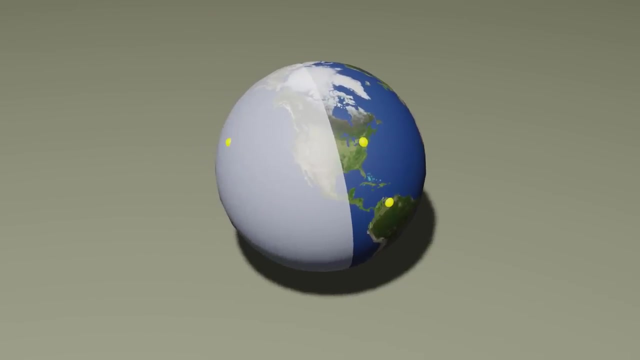 We can try an example: We pick five points at random and try some different hemispheres, And in this case we can eventually find a hemisphere that contains four of those five points. But will that always be the case? It turns out the answer is yes. 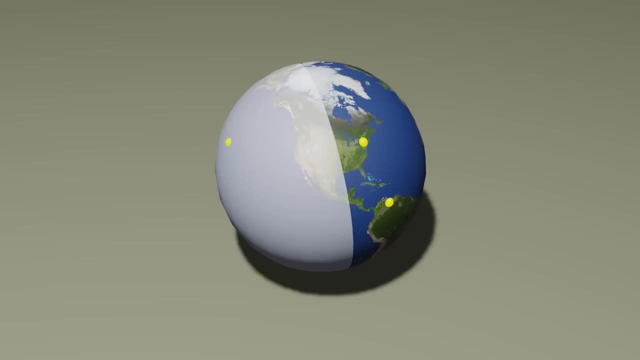 We can start by saying that with any two points on Earth, we can use those two points as the dividing line between the two halves. So that's the question. We can start by saying that with any two points on Earth, we can use those two points as the dividing line between the two halves. 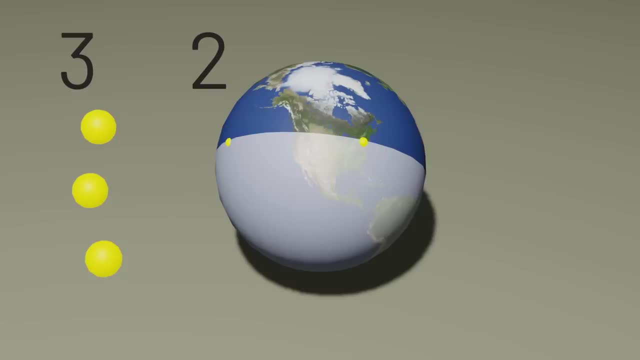 And if we can do this, then we can decide that there's no dismissal about the relationship between hemispheres. After that, we're left with three remaining points, each of which must belong to one of these two hemispheres. Do you see where the opportunity for the pigeonhole principle is? 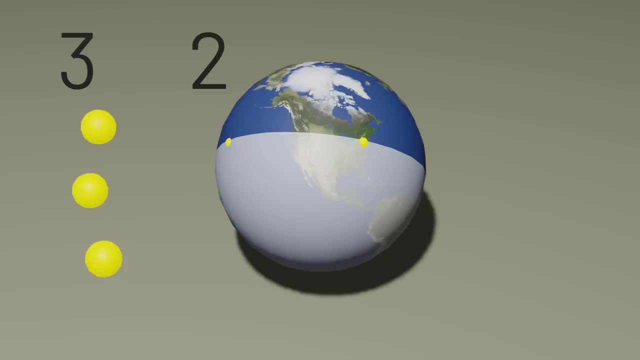 If we let the points be our pigeons and the hemispheres be our pigeonholes, look what happens. We have more points than hemispheres, so there must be some hemisphere that has at least two points, And if that hemisphere has a distance of at least one point, 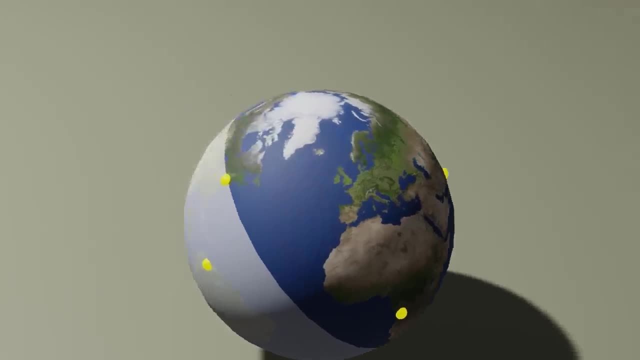 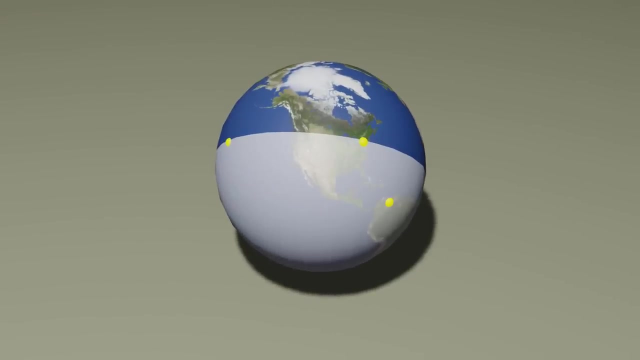 has at least two of these points, plus the two points on the dividing line, then it therefore contains four out of the five points on Earth. So for any five places on Earth, four of them will always be on the same half of the planet. proven. 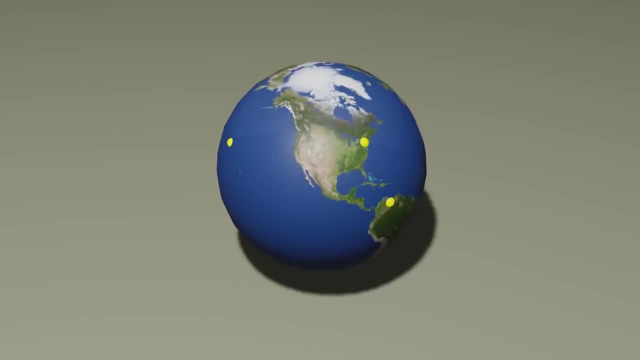 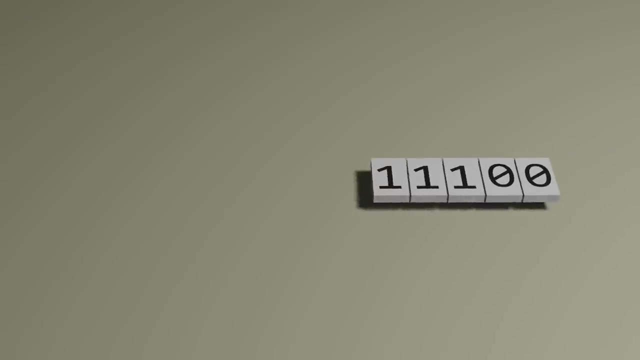 by the pigeonhole principle. And the pigeonhole principle isn't just useful for solving puzzles, it has practical computational consequences too. One natural extension of the principle has to do with compression, converting some longer representation of data to some shorter representation. There's a 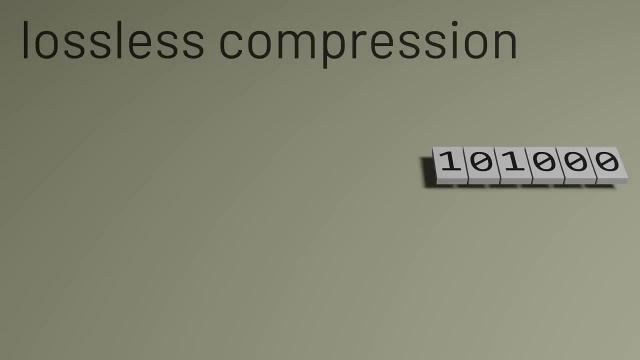 particular form of compression, called lossless compression, where, as the name suggests, no information is lost in the compression process. In other words, once we have the compressed version of the data, we can perfectly reconstruct the original information. Using the pigeonhole principle, we can. 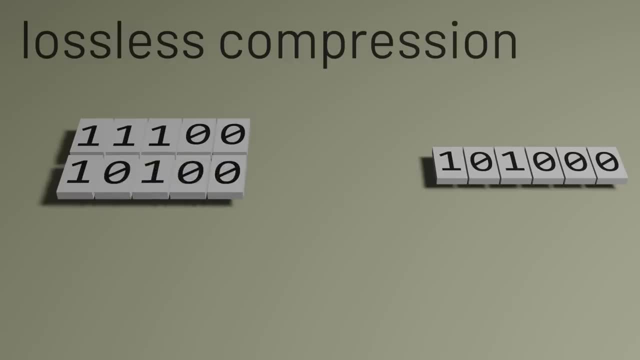 prove a thing or two that is actually a real thing. So, for example, if we were to prove that there is no way to have a lossless compression algorithm that always produces a smaller output for any given input, How can we do that? Well, if the input has n bits, there are 2 to the n possible values the input can take.